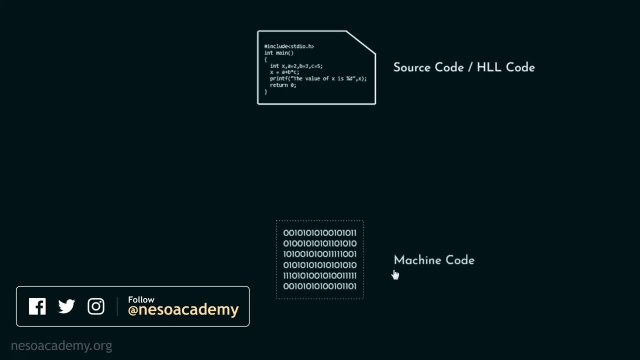 order to convert the human readable source code into the machine code, we need a language translator, And the language translator has got four different phases: The preprocessor, then the compiler, the assembler and finally the linker and loader. Now, after going through, 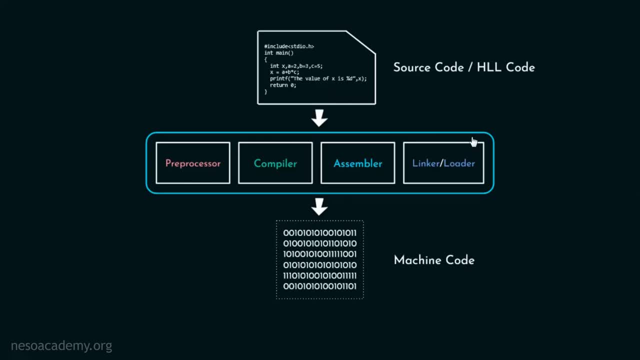 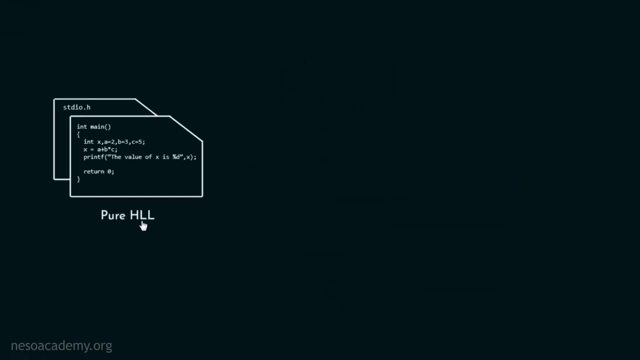 the preprocessor, the high-level language code gets converted into the pure high-level language code. Basically, the preprocessor will embed the required header files with the source code, omitting all the preprocessor directives. from that, Now this pure high-level 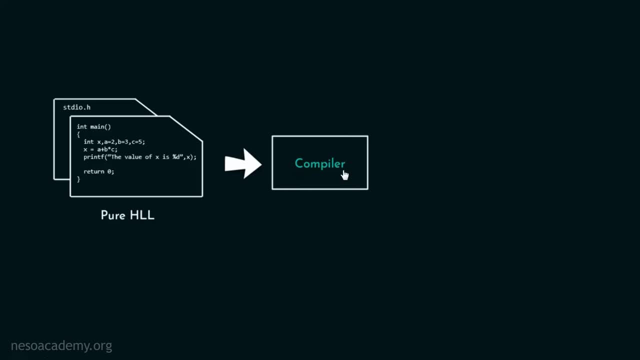 language code will be given to the compiler, which in turn will produce the equivalent assembly language code. Now, this much we have already observed in the previous session, So today we will take this pure high-level language code and observe how it goes through the various phases of. 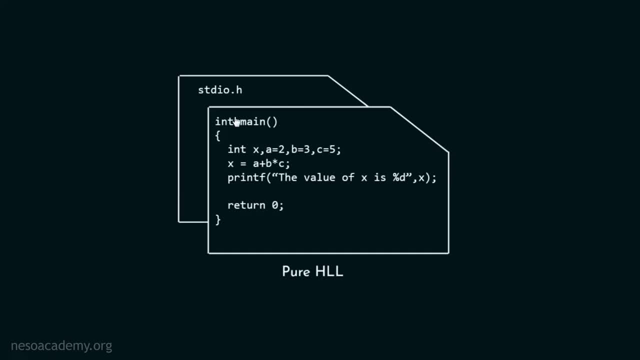 the compiler. Now, to be really honest, converting this entire piece of code will be a little time consuming. So what we will do instead of the entire code? let's consider this statement, that is, the arithmetic expression. We will observe how this expression goes through the 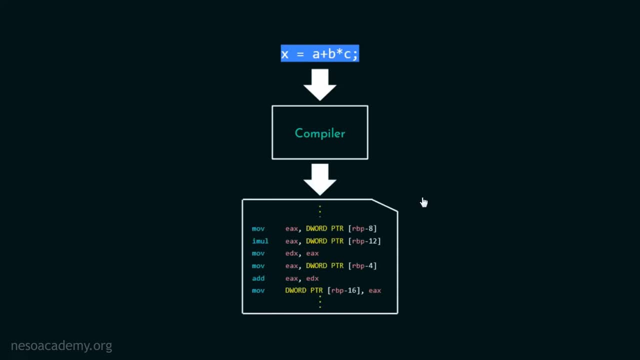 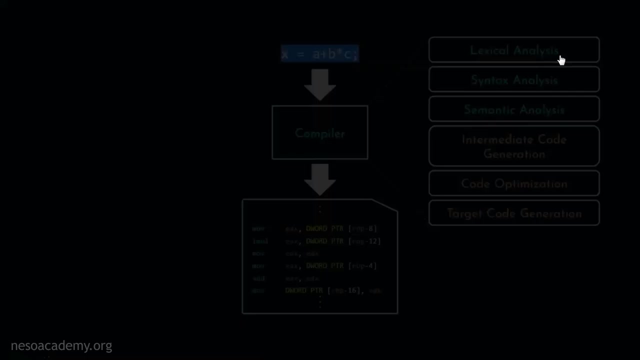 compiler and finally, how this particular assembly language code segment is produced. Basically, we will observe how this expression is treated by all the six phases of the compiler. Now coming to the first one, that is, the lexical analysis phase. here the entire process is taken care of by the lexical analyzer. 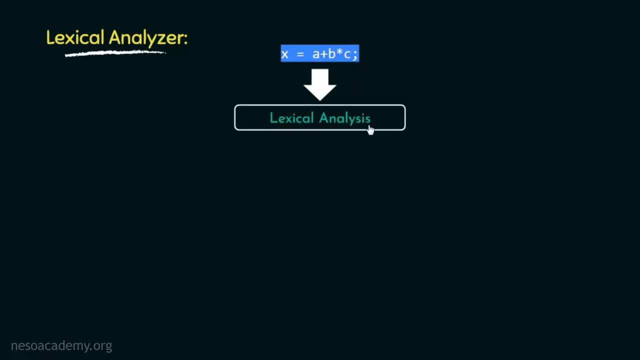 So here the expression is given to the lexical analysis phase and the lexical analyzer takes lexems as input. and the lexical analyzer takes lexems as input and the lexical analyzer takes puts and generates the tokens. Now lexems are similar to words with only one small difference, that is words individually. 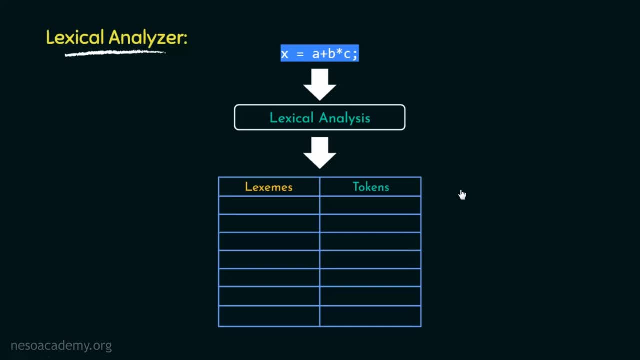 have their own meanings, whereas group of lexems in their entirety convey the meaning. For an instance, this word analysis means a detailed examination of anything complex in order to understand its nature or to determine its essential features. On the contrary, the lexical answer to this question is that words are in their own meaning and there are no definitions. 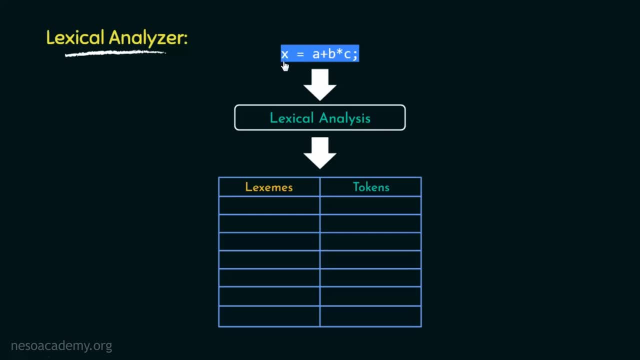 contrary, this x individually doesn't convey any meaning until we consider the entire arithmetic expression. Now, coming to tokens, these are actually the meanings of the lexemes. So if we traverse this statement from left to right, particularly in this statement, x is an identifier, then the equals symbol is an operator. to be precise, it is the assignment. 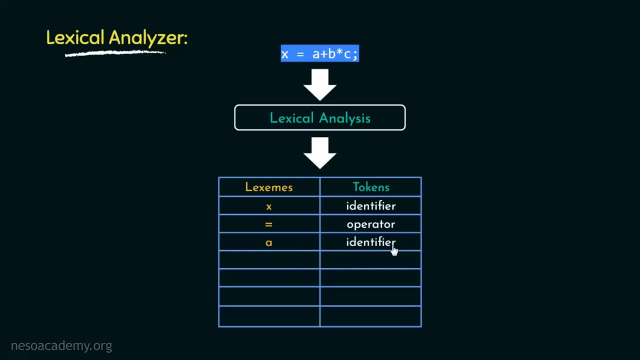 operator. thereafter, a is again an identifier, the plus symbol is an arithmetic operator, and so on. So this is the output of the lexical analysis phase, that is, the stream of tokens, and the job of the lexical analyzer is to find out the meaning of every lexem. 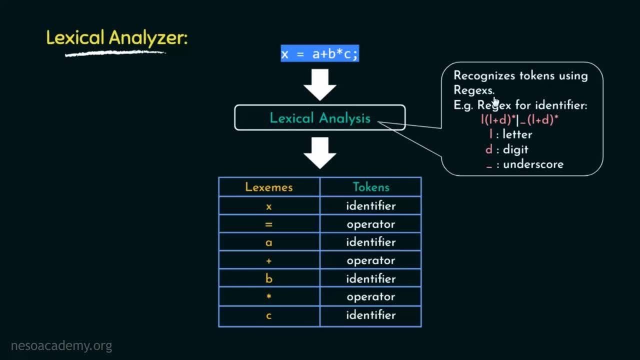 It recognizes the tokens with the help of regexes or regular expressions. Exempli gratia: this is the regular expression for identifiers, Where l stands for letter, d for digit, and this spatial character is the underscore. Now allow me to illustrate this using its equivalent finite automata. 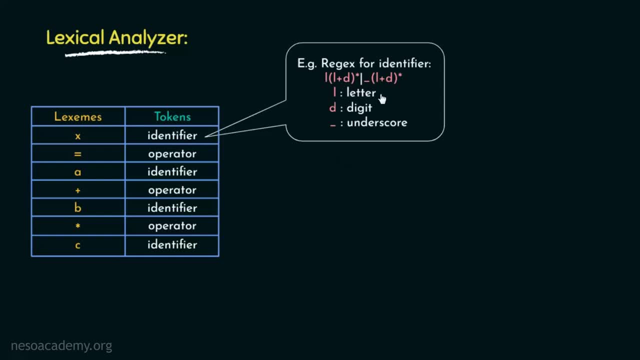 Observe, there are two regexes for identifier. Lets consider the first one. So from the initial state, that is, q- zero- seeing a letter, we will go to the next state, q1.. And from this one Seeing any number of letters. 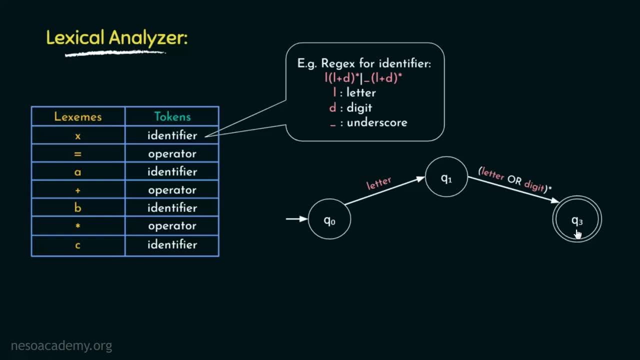 letters or digits, we will end up at the final state, that is, Q3.. Coming to the next form, starting from the initial state, if we see an underscore, we will move towards the next state, that is, Q2, thereafter seeing any number of letter or 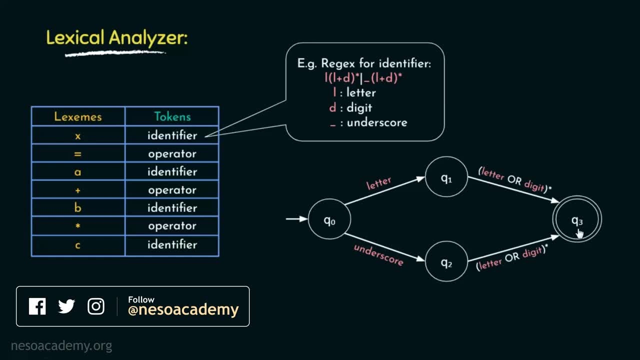 digits, we will end up at the final state, Q3.. Many of you may know this, that we cannot have an identifier name starting with digits, and this is the logic which rejects the identifier names beginning with digits. So for examining the lexemes, the lexical analyzer makes use of the type 3 or regular. 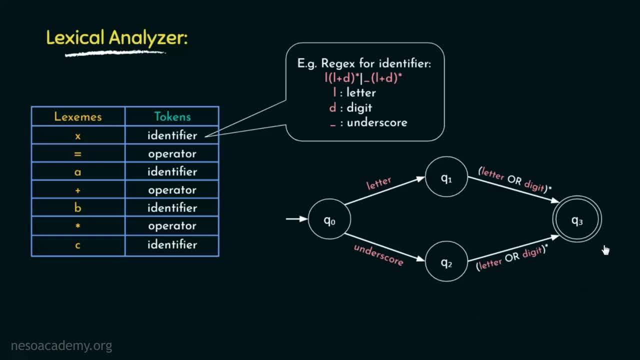 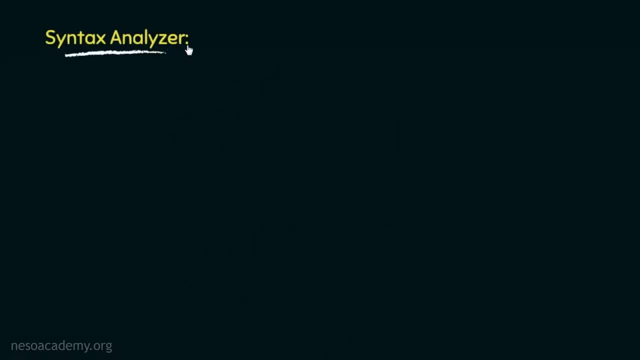 grammars of the family of grammars for formal languages. Now let's move on to the next phase. Here, the syntax analyzer, also known as the parser, is in control. The stream of tokens is passed to the syntax analysis phase- The syntax analyzer. 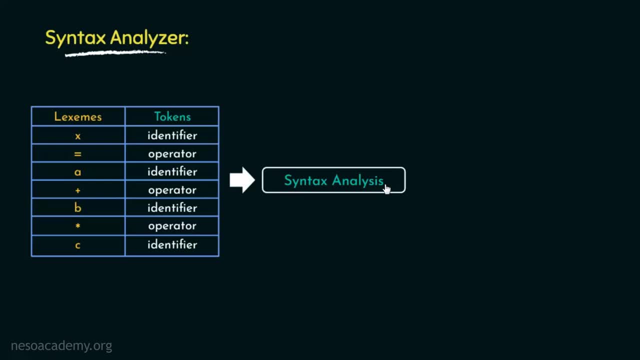 depends on the type 2 or context-free grammars For this particular expression. these are the CFG production rules that the parser will use in order to form the parse tree. Let me illustrate the formation of the parse tree. Consider the first production rule. 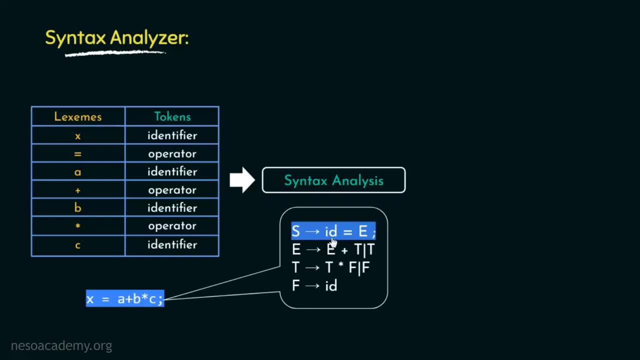 The start symbol s can be rewritten as id, equals e semicolon. It means an expression can be assigned to an identifier and the expression has to be followed by the statement terminator, that is the semicolon. So from s we can derive id, equals, operator e and semicolon. 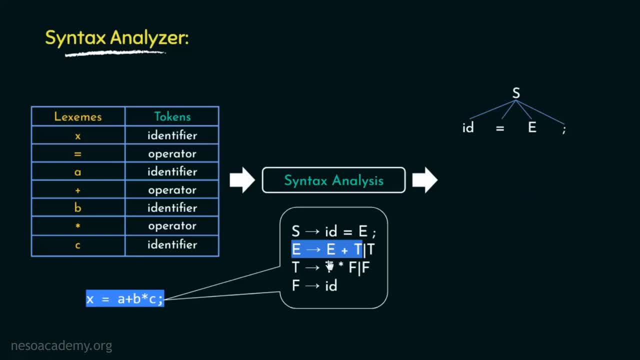 Coming to the next production rule, e can be rewritten as e plus t. That is, expression can be expression plus term. So from this e we can derive e plus t using the production rule. Now let's look at the next production rule. 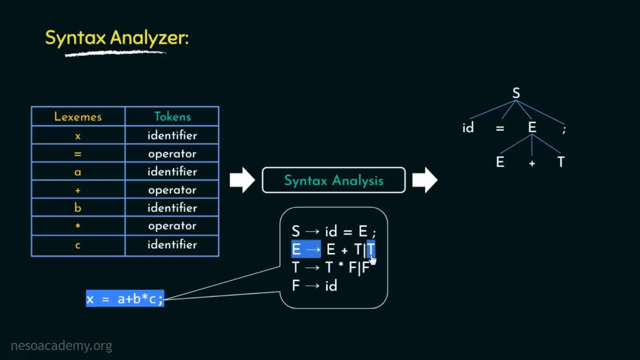 Now e can also be rewritten as t. That is, expression can also be a single term. So using this production rule, from e we can derive t. Coming to the next one, t can be rewritten as t into f. That means term can be a term multiplied by a factor. 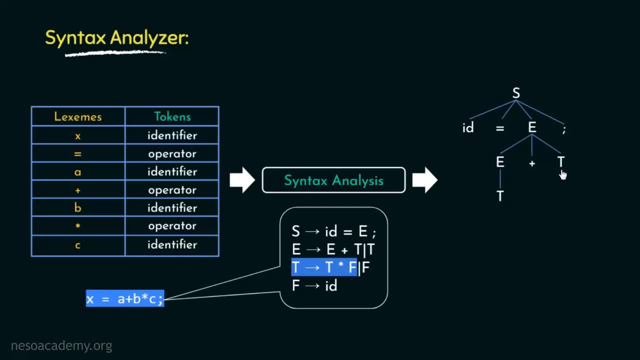 So from this t we will derive t into f. That is t, then the multiplication operator And then f. Additionally, t can also be rewritten as f, That is term can also be a single factor. So from t we can derive f in these two instances. 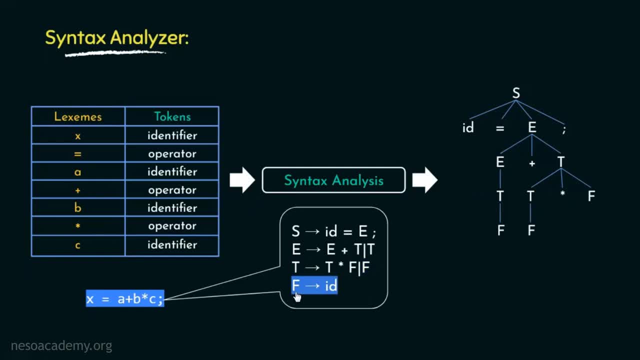 Finally, consider the last production rule. f can be rewritten as id, That is, factor is an identifier, And using this we can derive id from all these f's. So this is the parse tree. Now, before observing the yield of the parse tree, let me tell you a few things about this. 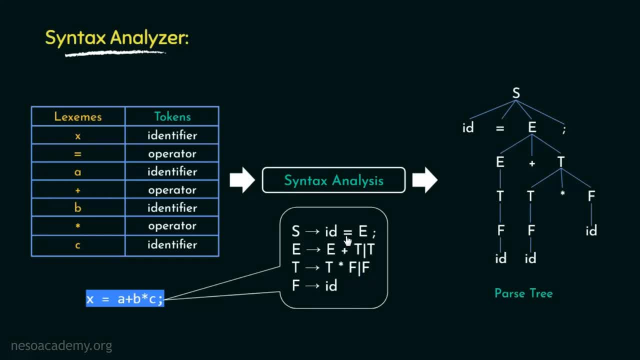 particular grammar Here, id, the equals operator, semicolon, the plus and the multiplication operators are the set of terminals And the ones in the uppercase, that is, s, e, t, f. these are the set of variables or non-terminals. Now, in order to find out the set of variables, we need to find out the set of non-terminals. So, in order to find out the set of non-terminals, we need to find out the set of non-terminals. 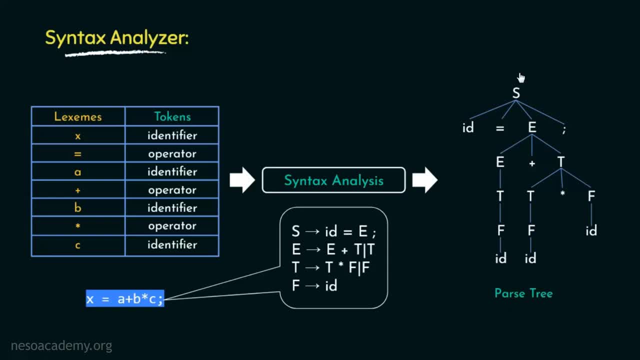 To find out the yield of the parse tree, we will have to traverse it top to bottom, left to right, taking notes of only the terminals. So let's begin. During traversal, this id is the first terminal that we encounter. Remember, top to bottom, left to right. 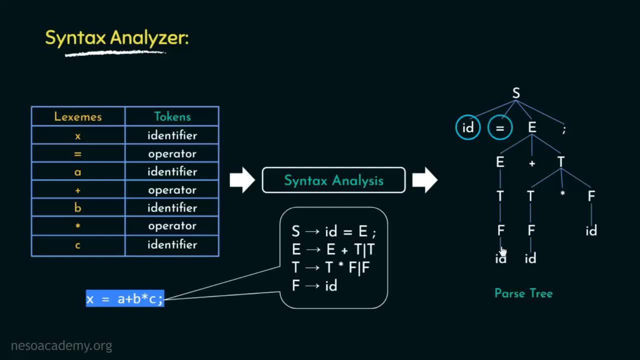 So the next one is this equals operator, next this id, thereafter this plus operator, then this id, Then this multiplication operator, after that this id and finally this semicolon. Therefore, the yield of the parse tree would be id equals id plus id into id semicolon. 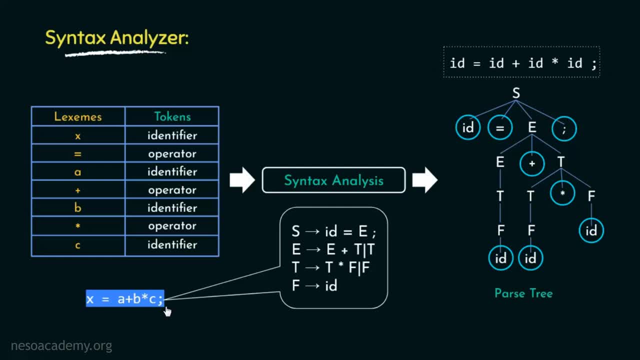 And since the yield of the parse tree and the expression are the same, the syntax analyzer will not produce any errors. So, in short, taking the stream of tokens, The syntax analyzer analyzes them following specific set of production rules and produces the parse tree. 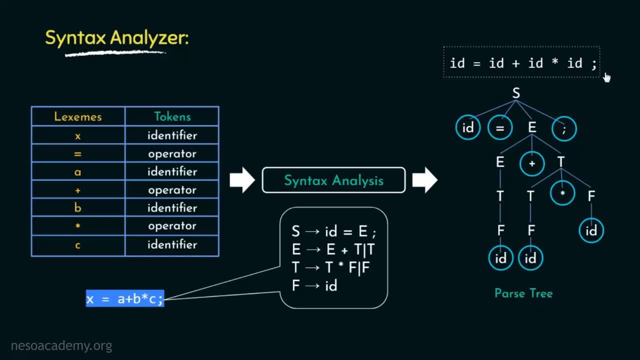 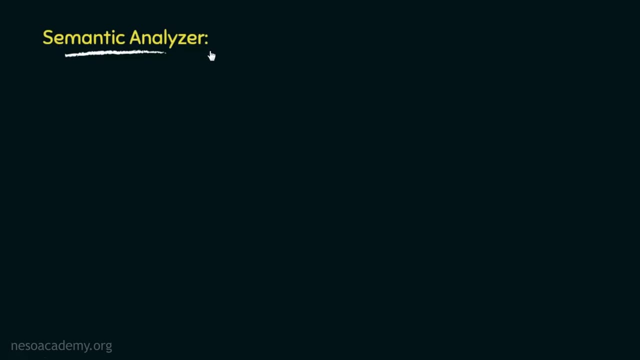 And if the yield of the parse tree and the provided stream of tokens are the same, then there is no error. Otherwise, there is some syntax error in the statement. Now let's move on to the next phase. In this phase, the semantic analyzer takes the control. 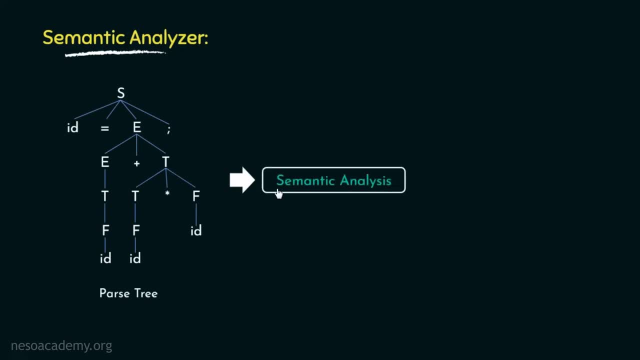 The parse tree produced by the syntax analyzer is given to semantic analysis function And the semantic analyzer in turn produces the semantically verified parse tree. Semantic analyzer is responsible for type checking, array bound checking and the correctness of scope resolution. Basically, it does the logical analysis of the parse tree. 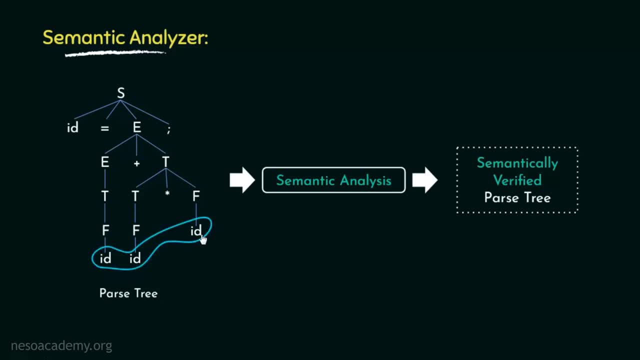 Like in this parse tree, these three identifiers can be constants, Whereas this particular identifier, because it is followed by this assignment operator, cannot be a constant. Here the semantic analyzer will examine whether the type of this identifier is variable. Semantic analyzer detects type mismatch, errors, undeclared variables, misuse of reserved words. 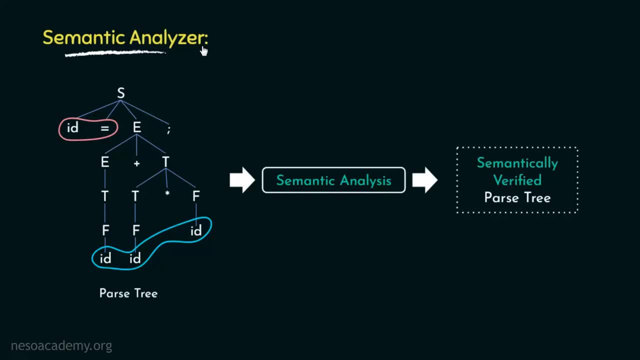 multiple declaration of a variable within a single scope, accessing an out-of-scope variable, mismatch between actual and formal parameters, etc. In simpler terms, Semantic analyzer looks for the meaningfulness of the parse tree and verifies that. Now the next phase is handled by intermediate code generator. 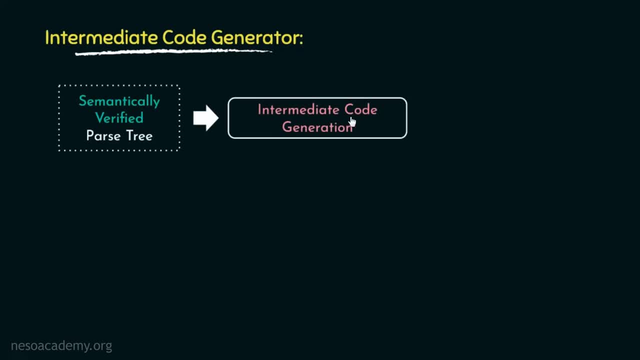 The semantically verified parse tree is given to the intermediate code generation phase, where the intermediate code generator in turn produces the intermediate code. So this was our parse tree And this is the yield of the parse tree, which is similar to the pure high-level language. 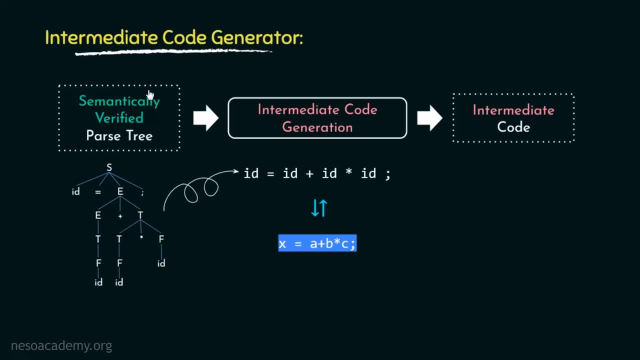 expression. After being semantically verified, the intermediate code generator will produce the intermediate code. Here we are using the very popular intermediate code, that is, the three-address code, TAC. Now, if you observe this parse tree carefully, the precedence of the operators are visible. 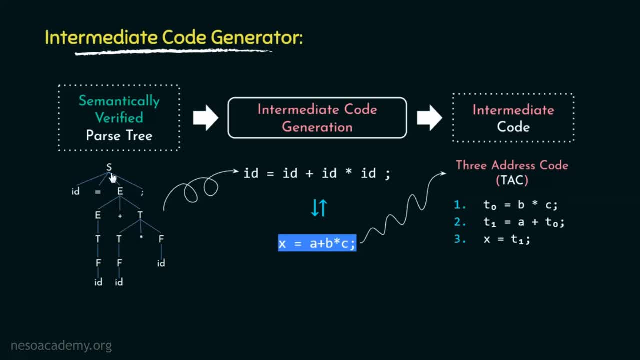 here. if we look at the tree from bottom to upwards, So at the lowest level, the multiplication operator is there And therefore this would be performed at first. For this, the intermediate code generator will create this and assign the result of bxc to it. 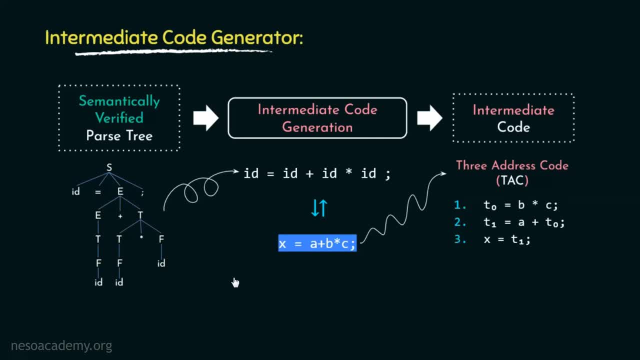 Comes to the next level. The result of this is being added with this identifier Which in the expression, is A. Therefore, in the intermediate code, the result of a plus T0 is being assigned to another temporary variable, T1.. And finally it is displayed as t0.. 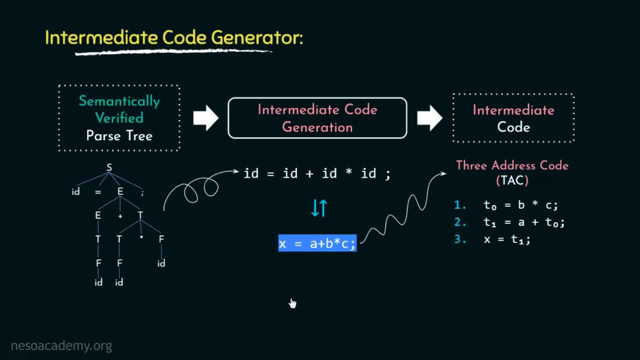 Look again now. Finally, in the last level, the result of the expression is being assigned to this identifier which in the arithmetic expression is the variable x. So in the intermediate code, t1 is being assigned to x. Now this intermediate representation of the code is called 3-address code, because if you 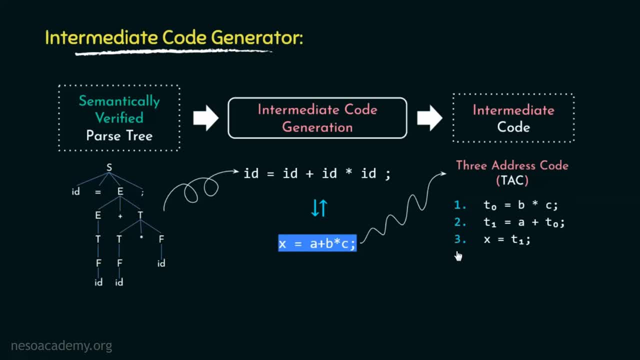 observe all the statements in here, at most they have 3 addresses in them And by saying address we are mentioning the addresses of these variables. Now till this phase. it is called the frontend because, taking this intermediate code, if we want to generate the target code which is specific to the platform, all we have to 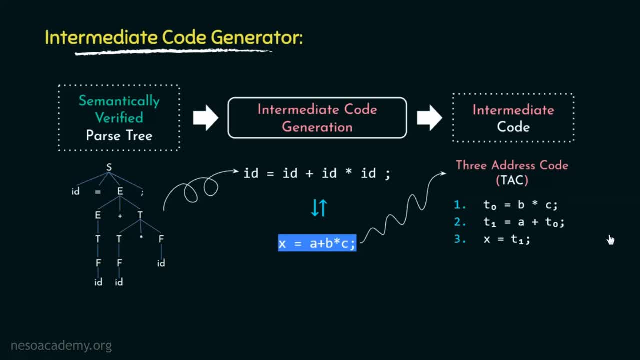 do is modify the next two phases, that is, the backend, according to the platform which we want to produce our target code. for Now, let's move on to the next phase, shall we So? here, the code optimizer is in control. 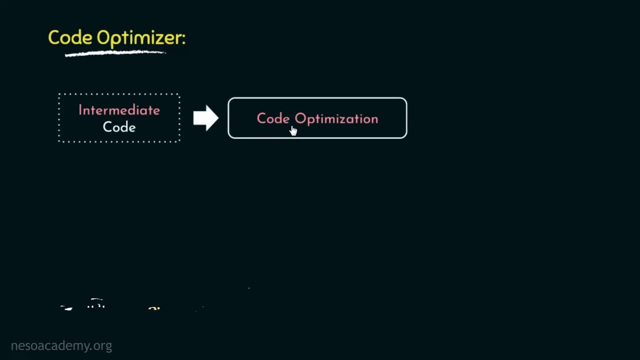 Basically, the intermediate code is provided to the code optimization phase. there, the code optimizer in turn generates the optimized code. Now, code optimization can either be machine dependent or machine independent. We will observe them in details in due time. For now, for the sake of understanding, let me illustrate the optimization procedure. 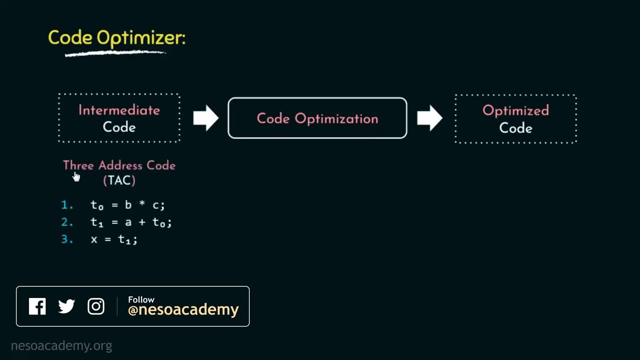 So, as you can observe, The initial code, that is, the 3 address code, had 3 statements. In the first one, t0 is being assigned, with the result of b into c. Then in the second one, t1 is being assigned with the result of a plus t0.. 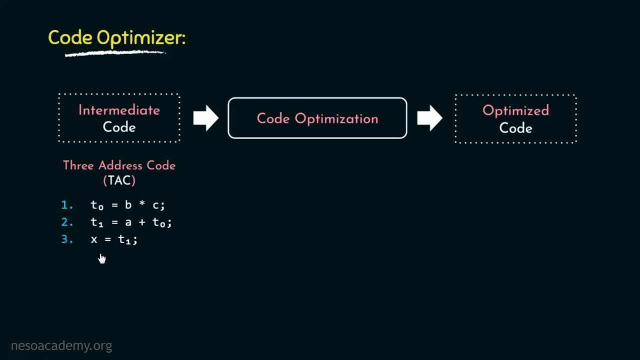 And finally, in the third one, we are assigning t1 to x. Now, if you observe carefully the second and the third statements, here, instead of t1, if we assign a plus t0 directly to x, It will reduce the length of the code. 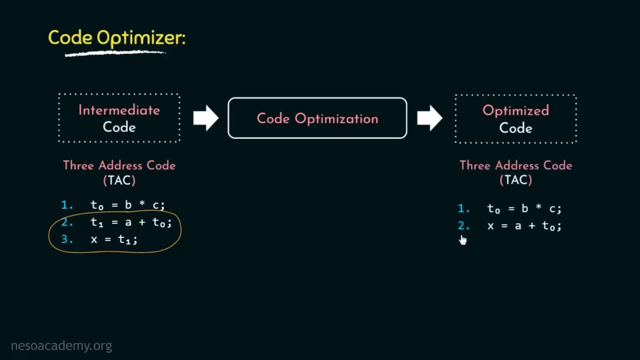 So the optimized code will have only two statements And, in a nutshell, this is exactly what the code optimizer does: It optimizes the intermediate code. Next up is the target code generator, So the optimized code is given to the target code generation phase, which happens to be. 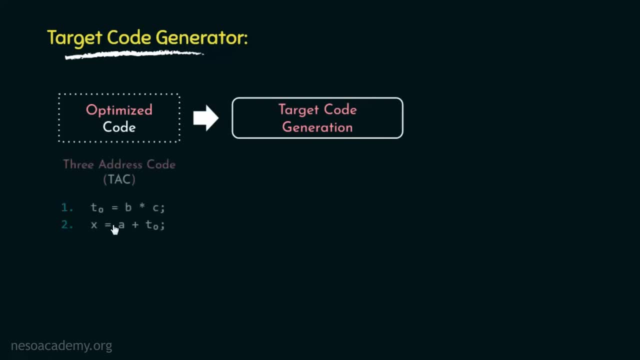 the last phase of the compiler. Now, taking this optimized code, The target code generator Will finally produce this assembly code segment. Allow me to walk you through this code segment. Here, in the first line we have mov. That is the mnemonic for moving. 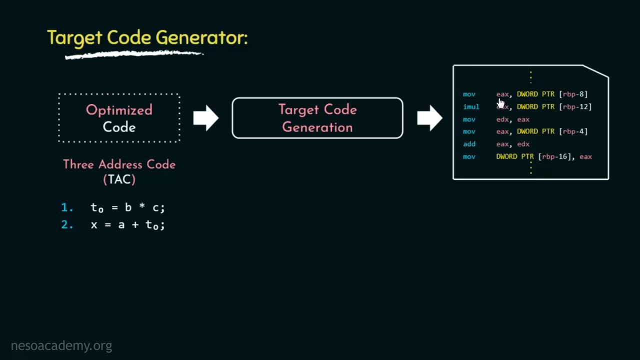 Then we have eax. Now eax is actually the extended version of the ax register, Which is a combination of ah and al. Ah can store 16 higher order bits And al stores remaining 16 lower order bits, So eax can actually store 32 bits. 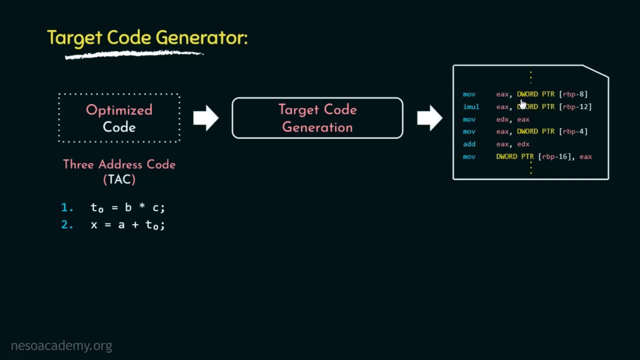 It is actually the accumulator register. Next, we have dwordptr, That is the data word pointer, Which is pointing at the register based pointer rbp With a scaling factor of minus 8.. Basically, this pointer is pointing to the variable b And, using this entire command, the value held by variable b is being moved to the eax register. 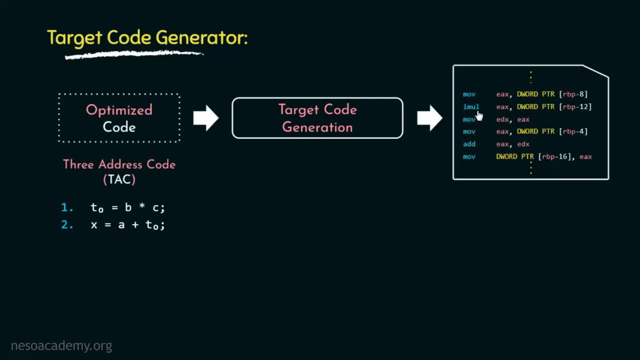 Now this iml Is the mnemonic For sign multiplication. Dwordptr rbp minus 12 is pointing to the value stored by the variable c And using this command, the value stored in variable c is being multiplied with the value stored in the register eax. 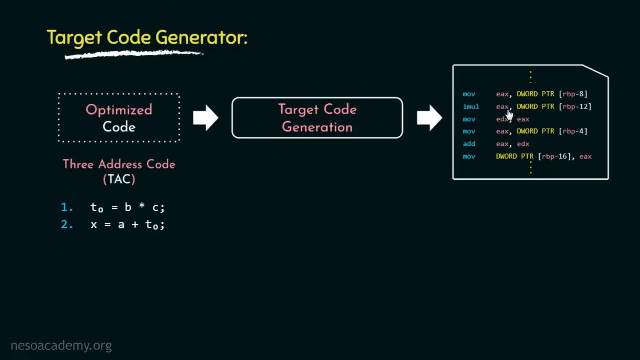 And the result is also stored in the eax register. Basically, by the end of these two commands we will have the result of b into c in the accumulator. Coming to the next command, Here The contents of the eax register are being moved to another register, edx. 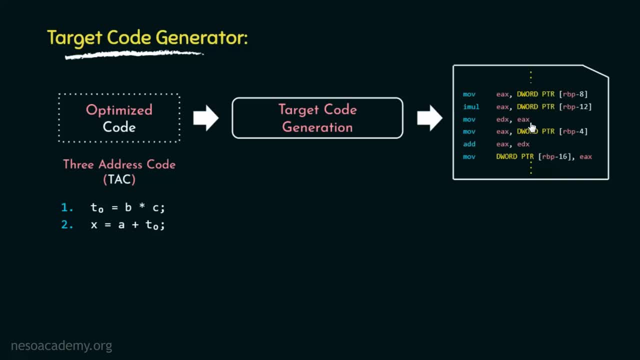 Which also is a 32-bit register Similar to eax, edx also has two different 16-bit segments, Where the higher order 16 bits are to be stored in dh And the lower order 16 bits will be stored in dl. Now, in the next command, we are moving the data word pointed by register based pointer. 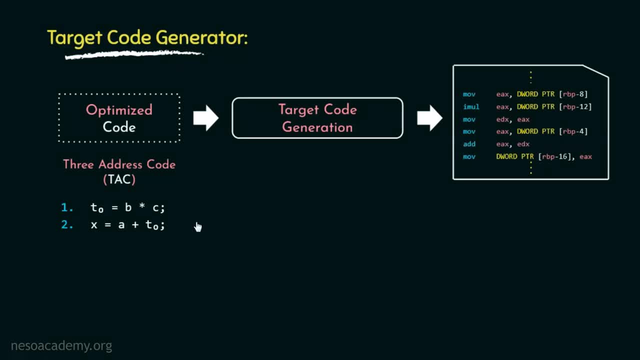 with the scaling factor minus 4.. That is the content of the variable a into the accumulator. Thereafter in this command we are adding the contents of the register eax and edx And also storing the result in the eax register. That is the accumulator. 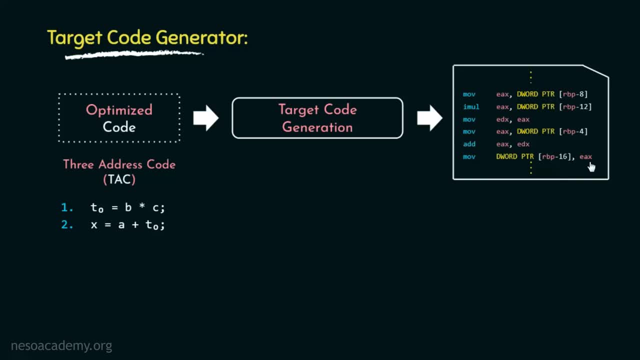 Finally, we are moving the content of the eax register to the address pointed by the data word pointer rbp minus 16.. Which is actually the address of the variable x. So, After execution of these commands, We will have the calculated value in the x. 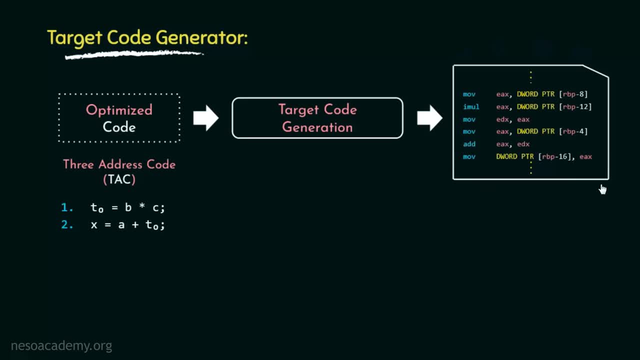 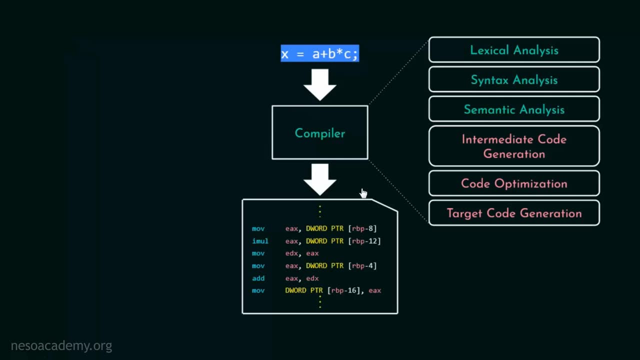 So this is the meaning of this assembly language code segment. So this is how that arithmetic expression of our pure high level language code finally gets translated into this assembly language code segment. after going through all these phases, Now let's observe the tools using which we can practically implement various phases of.